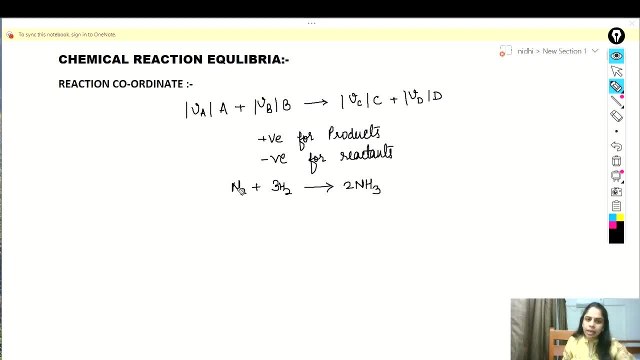 and H3.. So here you can see. the statuometric number of N2 is minus one's reactant. That's why we have minus negative sign Here. it is minus three and two. So this is how you can. we can find the find the statuometric number for individual components and for any inert gas statuometric number. 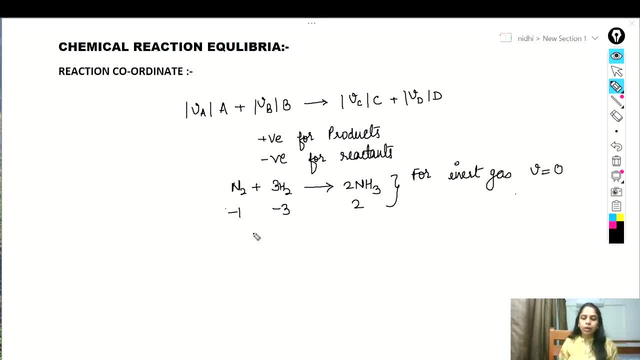 Guess Stichiometric number is 0. So for any reaction the change in the number of moles of any component present in any side are directly proportional to the its stoichiometric number. So apply to a differential amount of reaction this principle: provide d n i upon mu i is equals to. you can write: 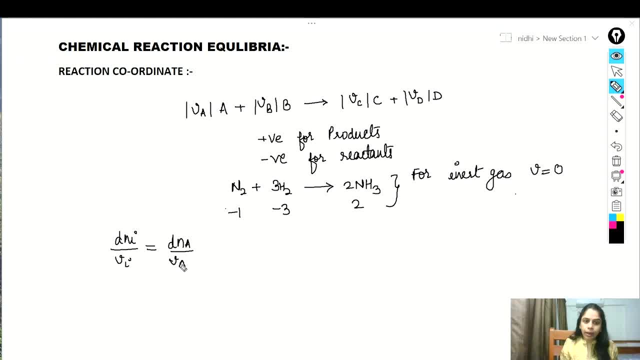 for individual components: mu a, d n b upon mu b. So this is your number of moles and this is a stoichiometric number: d n, c, mu c and d n d. mu d is directly is equal to the differential change in reaction coordinate. Here it is a epsilon, and epsilon is what 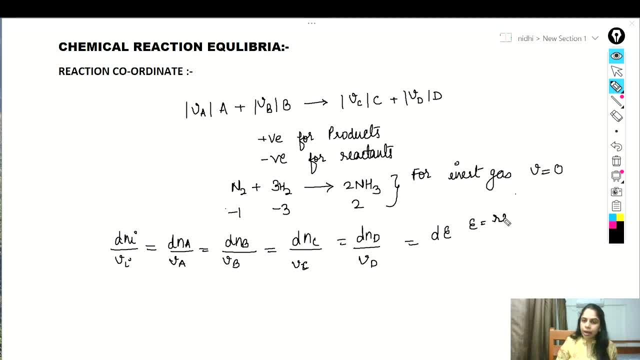 It is a reaction coordinate. epsilon is reaction coordinate. so we this quantity we identify as a reaction coordinate, right and the what is d? epsilon is differential change in the reaction coordinate. so this is what differential change in the differential change in reaction coordinate, in reaction coordinate. so from here what we have, we have relationship that d and I. 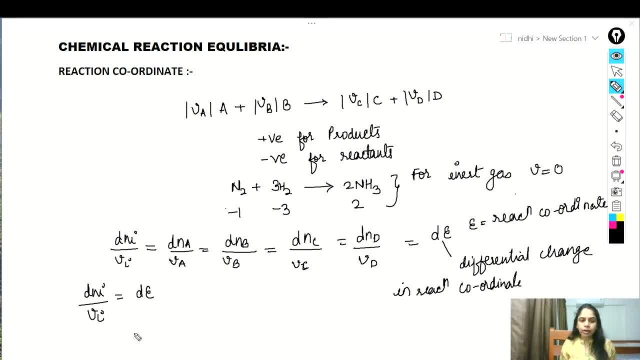 stoichiometric coefficient d, epsilon right. so rearrange this. so what we have, d and I is equals to mu I, d, epsilon. right now. just integrate this equations, integrate, integrate the above relation, above equation. so we integrate from and I, not the initial number of moles, to the final. 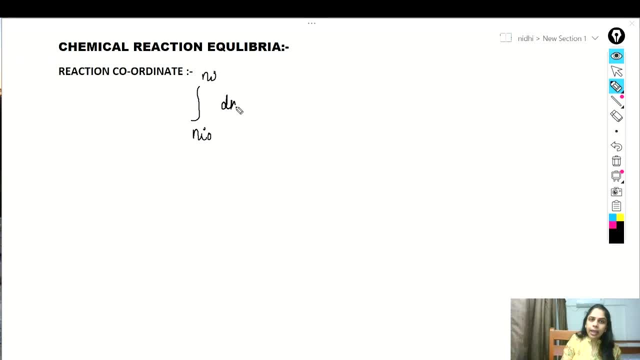 number of moles of any species, I, d and I is eqaussed to. so initial reaction is zero and then upsulate apps alone means how far it's now. then this energy also means how the reaction is proceed. okay, epsilon means how far the reaction proceed. So a reaction coordinate. 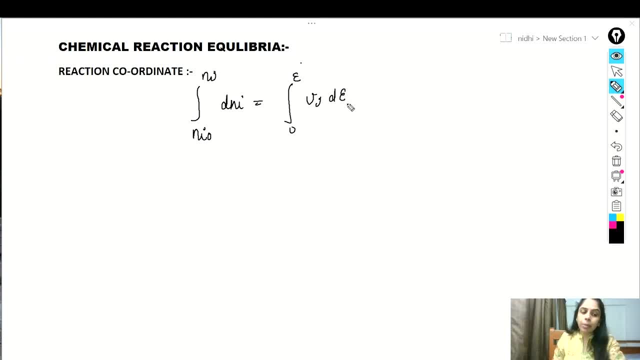 or extent of reaction is a quantity that measures the extent in which the reaction proceed. right, So reaction coordinate. here you can write: this is a reaction coordinate, so this is the quantity, right, this is the quantity that measures the extent in which the reaction proceed. or we can: 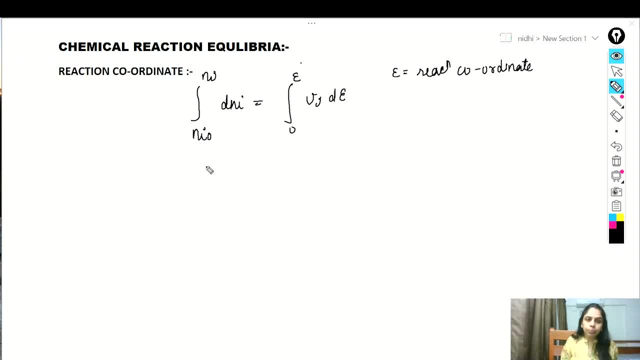 say how far the reaction is proceed. So when you integrate this, what we get n i minus n i naught is equals to nu i epsilon. So rearrange again this: n i naught plus nu i epsilon. Let's take this as the equation number one Now. summation of overall summation. 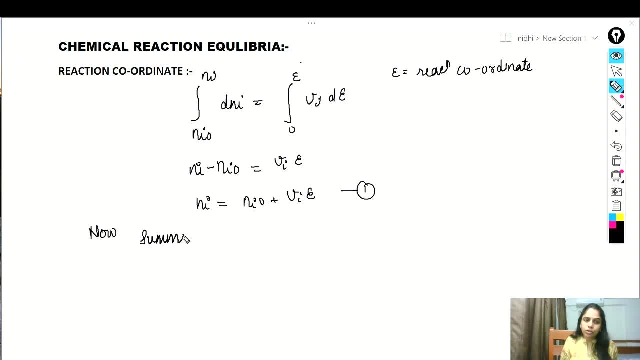 of the reaction is equal to n i minus n i naught. So let's take this as the equation number one: Species: summation of overall species. So capital n is equals to summation of total number of i species. if there are i species are present, right Then i initial number of moles plus epsilon of. 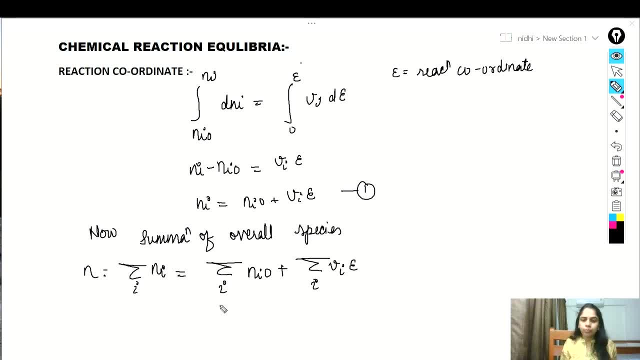 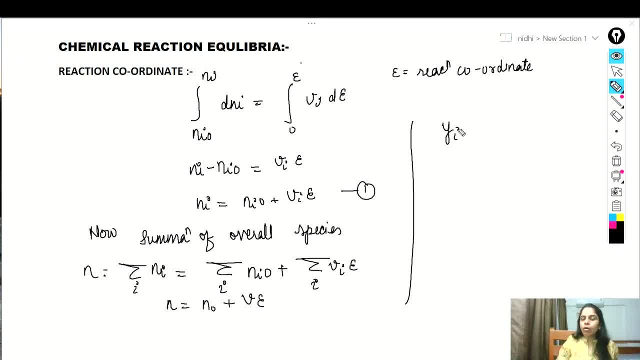 Now we can. we know that that y, i or x? i, the number of mole fraction and liquid and vapor phase is given by initial number of moles of that particular species upon total number of moles. So now we have all the values. Let's take this as the equation number two. So we have n? i is n i naught, initial number of moles of.